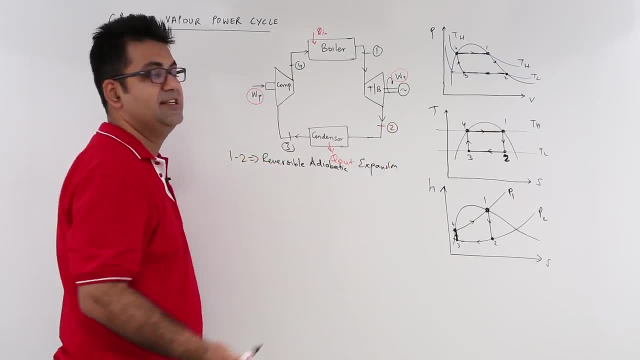 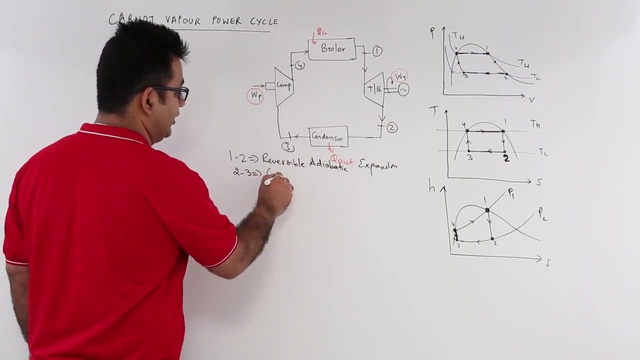 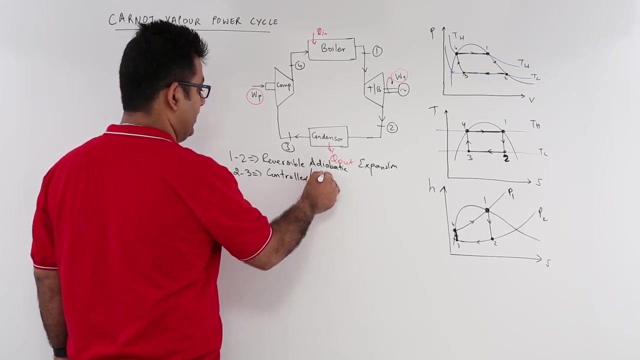 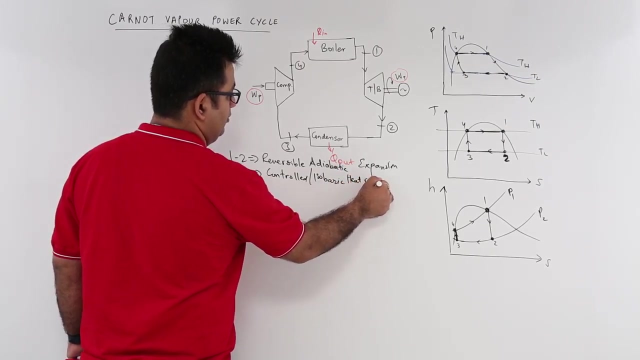 Reversible adiabatic expansion, So it has some work. output 2 to 3. This is controlled condensation, So we keep the pressure almost same. So I would say isobaric, Okay, Isobaric heat rejection. 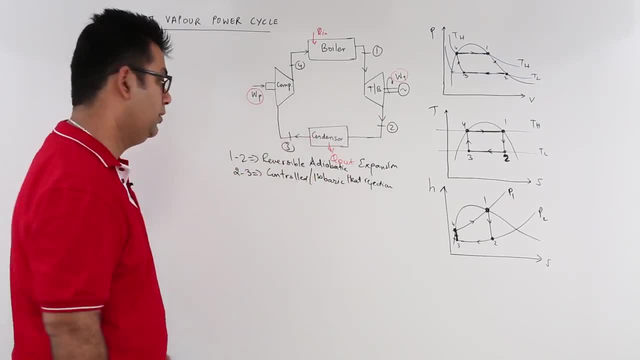 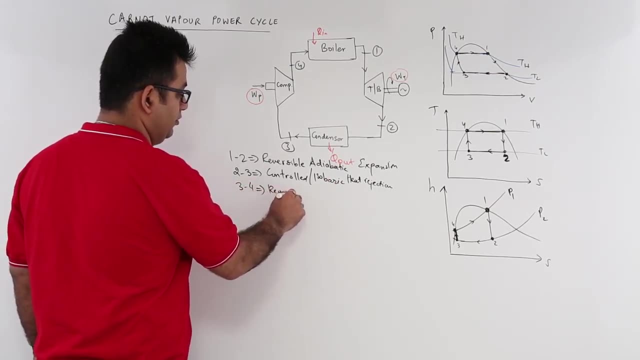 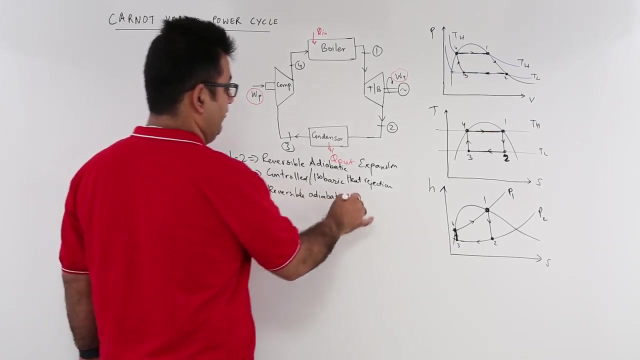 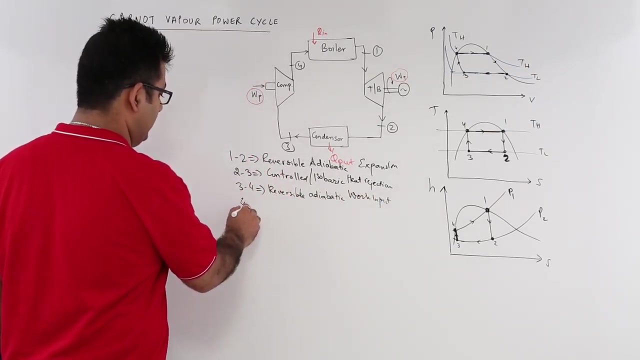 Okay, We will discuss these three diagrams one by one. Then 3 to 4.. This is reversible adiabatic work input. Okay, And then 4 to 1 is basically isobaric or controlled heat adhesion- Heat adhesion. 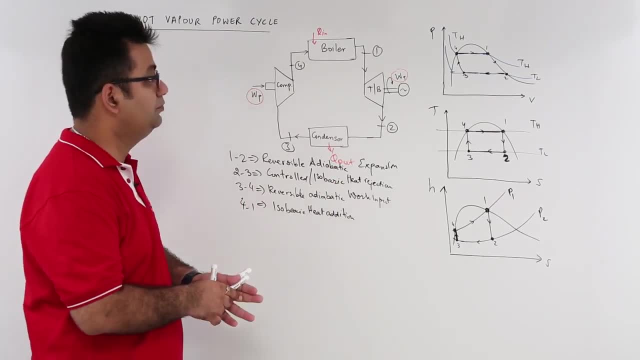 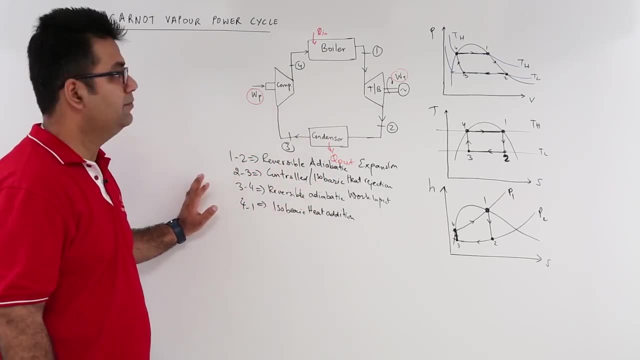 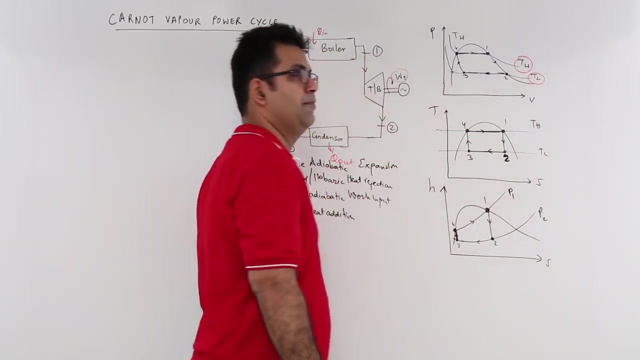 Okay. So if you look at these diagrams now, There are two temperature limits and two pressure limits under which this cycle is working. So the first, let's talk about temperature. So it operates between TH and TL. Okay, 1 to 2.. 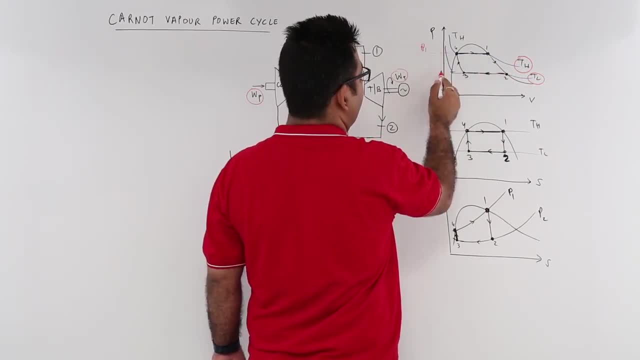 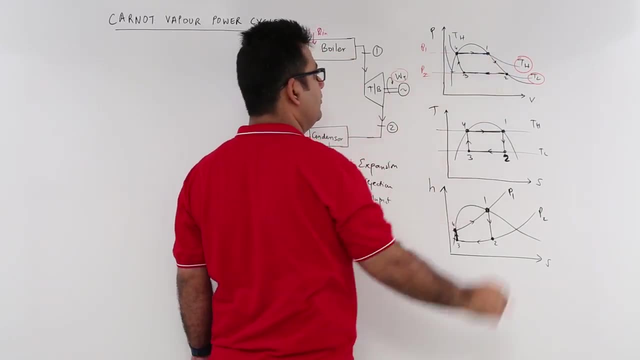 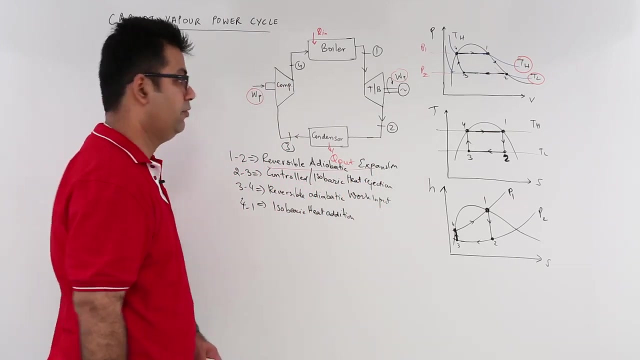 1 to 2.. Your pressure in the turbine inlet: The turbine inlet is P1 and the turbine outlet is P2.. Okay, So your pressure falls from 1 to 2.. And temperature falls from TH to TL and the process followed is a reversible adiabatic expansion from 1 to 2.. 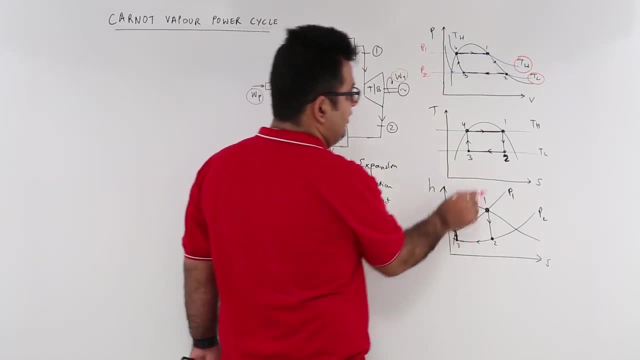 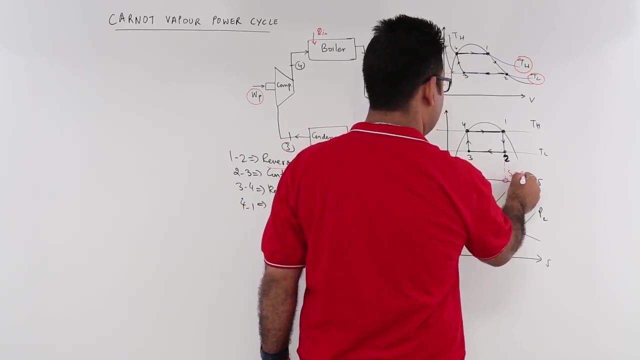 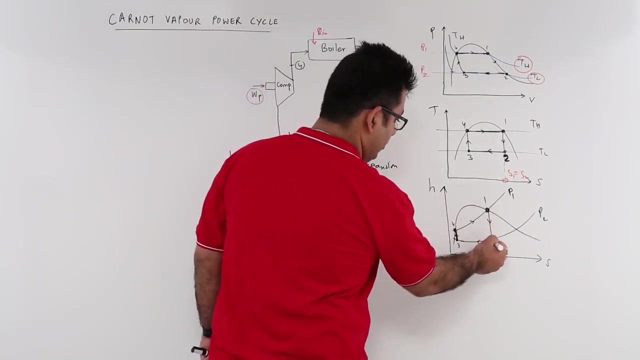 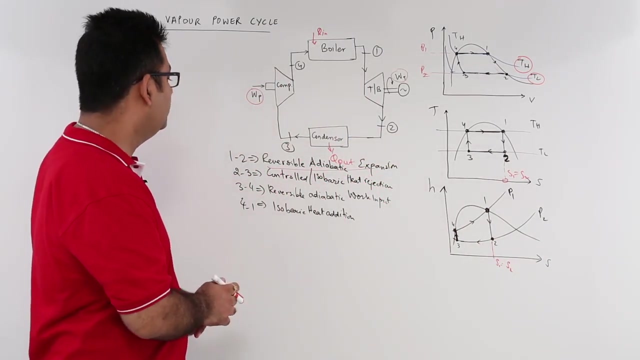 If you plot this one onto the TH plot, This is a vertically straight line which shows that S1 is equal to S2.. Same entropy, Okay. And similarly on the TH plot, which shows S1 is equal to S2.. Okay, Then let's move to 2 to 3, which is isobaric heat rejection. 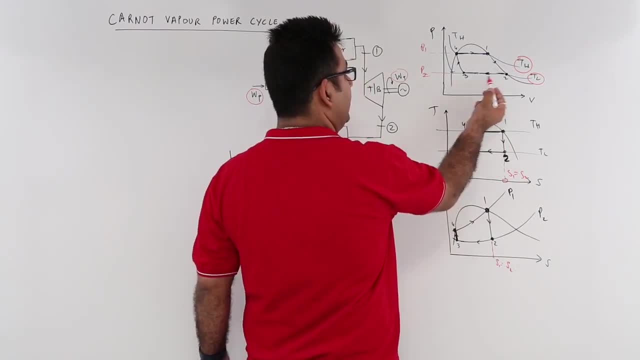 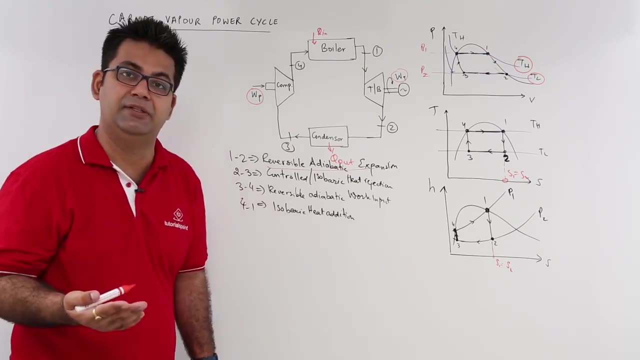 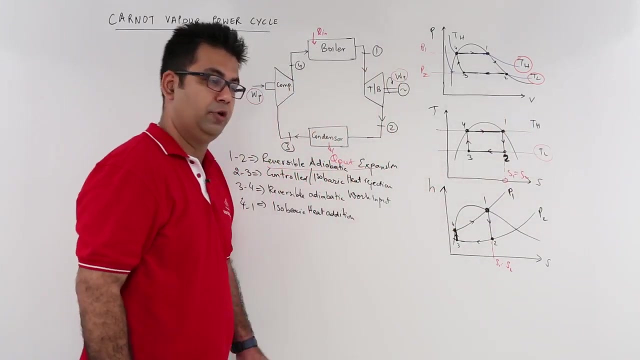 So if you go from 2 to 3 you are working on the same pressure- P2.- And there is some heat rejection Means condensation takes place. So whatever heat that we lose is the latent heat at constant temperature. So 2 to 3 is a isobaric, or you can say you lose latent heat. 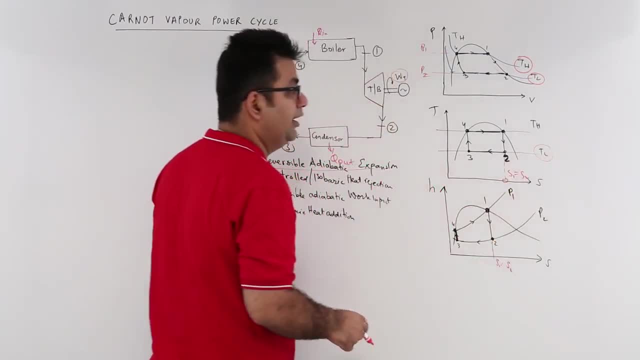 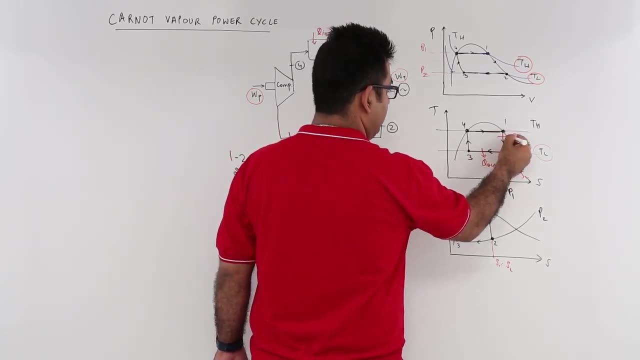 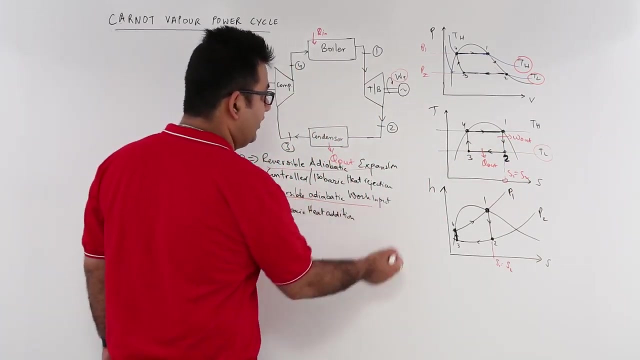 So you remain at constant temperature. So this is 2 to 3.. So you lose some heat from here And this is some work output or turbine work. Okay, Then, from 3 to 4 you have reversible adiabatic work input. 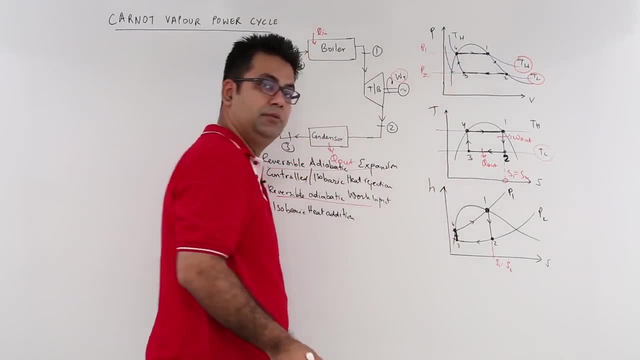 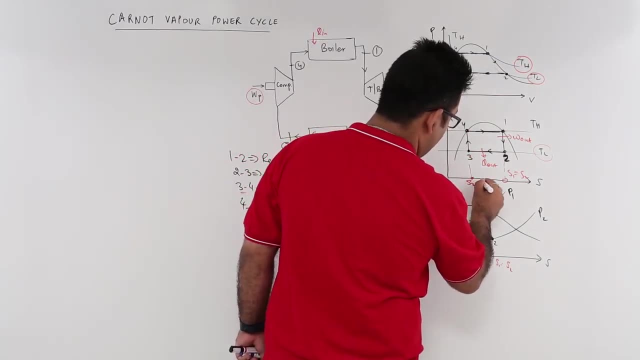 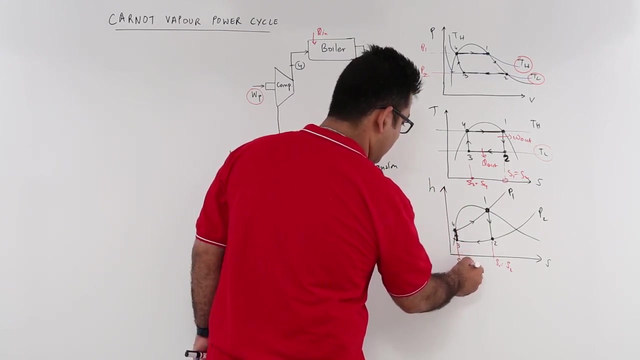 So now 3 to 4. you are compressing it, You are pumping it. Okay, So this is 3 to 4.. Again, it shows that the entropy at 3 and 4 is same, Okay. And similarly, over here, S3 is equal to S4.. 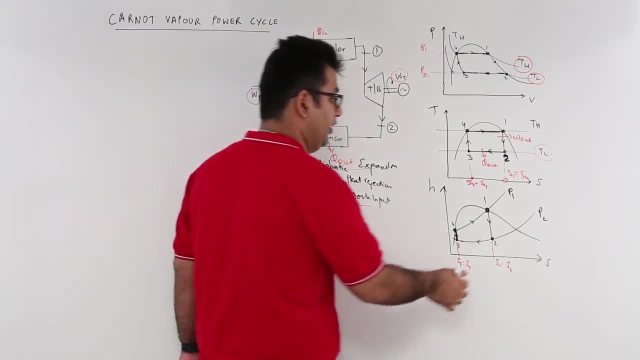 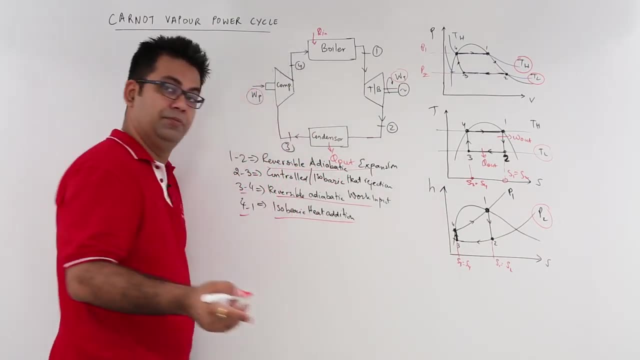 And the isobaric operation 2 to 3 is also evident over here. Same pressure, 2 to 3.. Okay, Now let's come to 4 to 1.. It is isobaric heat adhesion. So 4 to 1, you put some heat into it which is at same pressure. 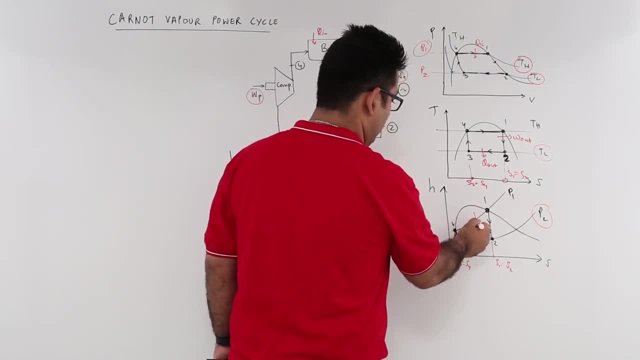 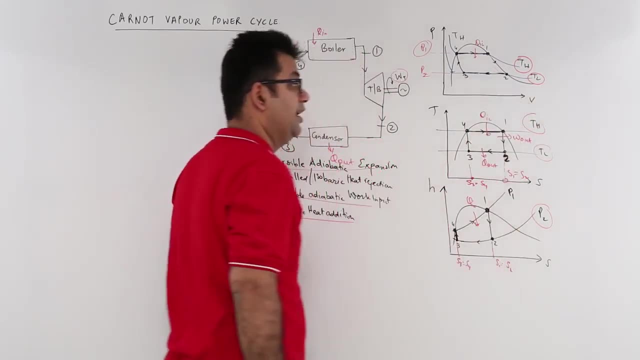 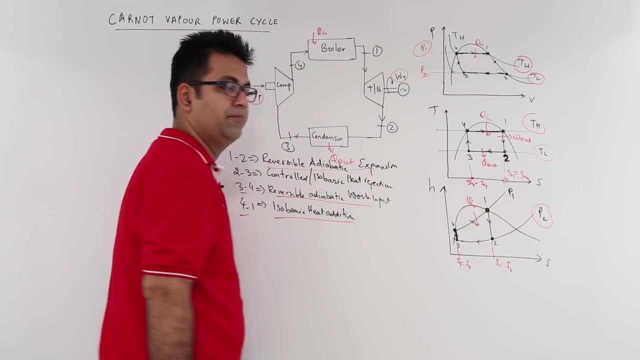 Okay, And this also shows same pressure. Okay, And this also shows same temperature, as we are adding the latent heat Right Now, how much heat is added? Either you use the TS plot, Okay, Or you use the HS plot. If you use the HS plot, 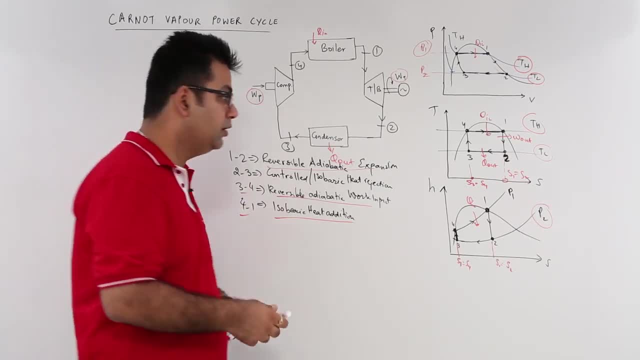 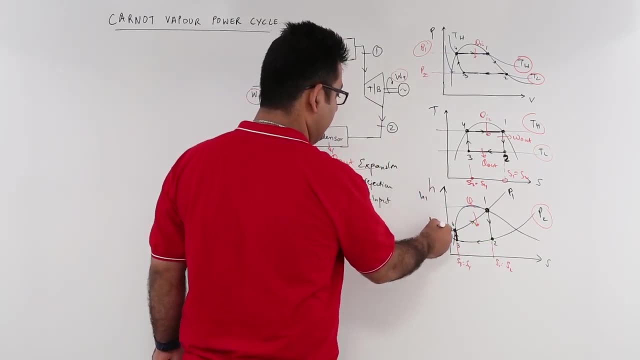 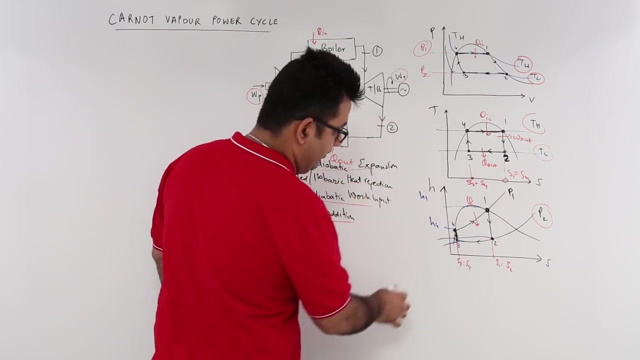 The amount of heat added would be the difference between these two entherpies, H1 minus H4. straight away, get these values from the Mollier chart And the amount of heat rejected would be the difference between H3, H2 and H3.. 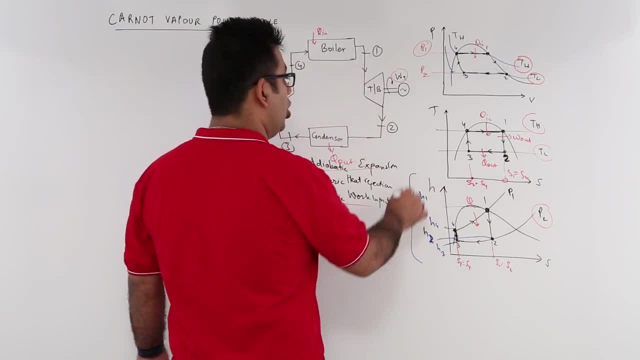 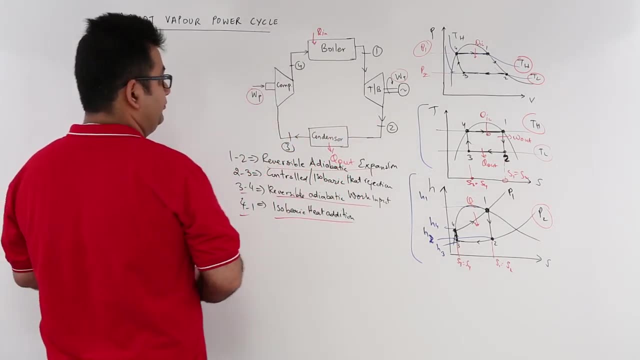 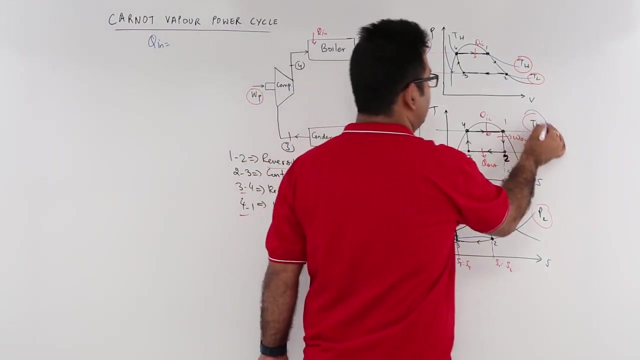 So either you can use this chart or you can use this chart Because the area below the TS chart is the heat added, That is, the heat interaction. Okay, So if I talk about the heat input, that is Q in, That is taking place at TH. 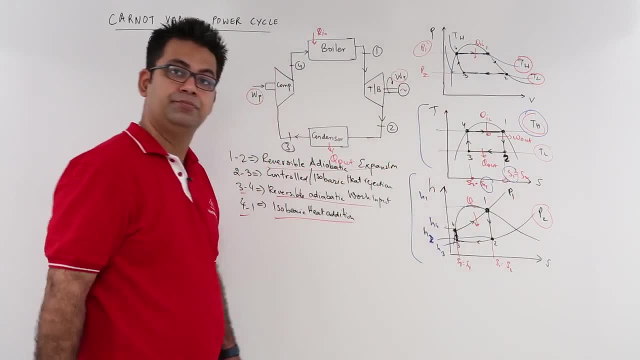 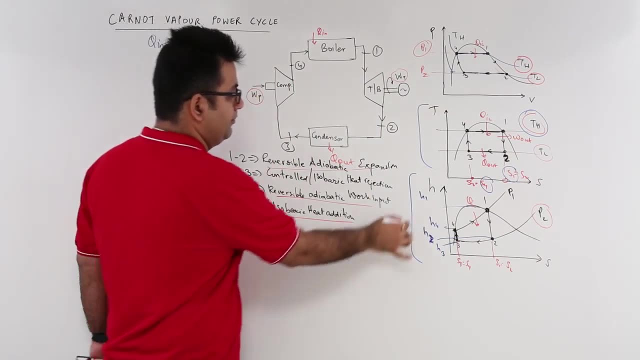 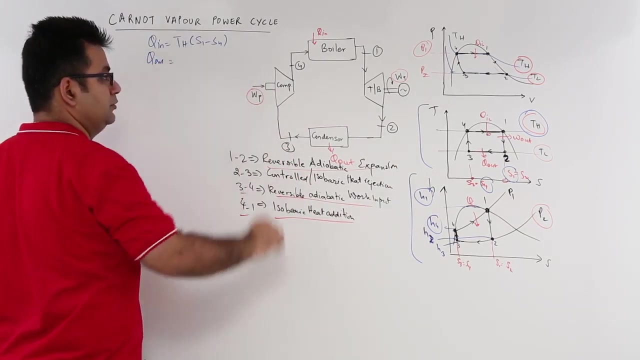 So TH into S1 minus S4. You will have TH into S1 minus S4, or simply H1 minus H4.. Okay, Then Q out. This takes place at TL. TL into S1 minus S4, because S2 is equal to S1 and S3 is equal to S4.